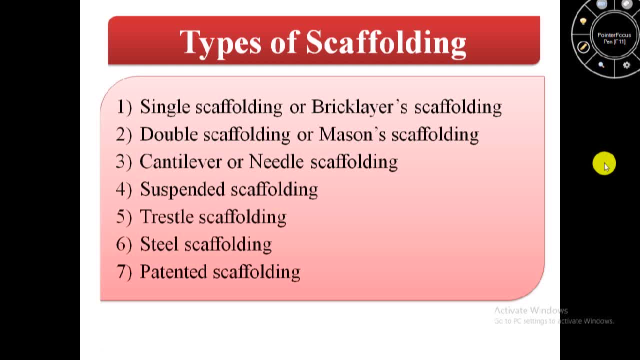 cantilever or needle scap folding, suspended scap folding, trestle scap folding, steel scap folding and patented scap folding. So in this video we will discuss all these types of scap folding one by one, in detail. So firstly we will discuss about single scap folding, which is also 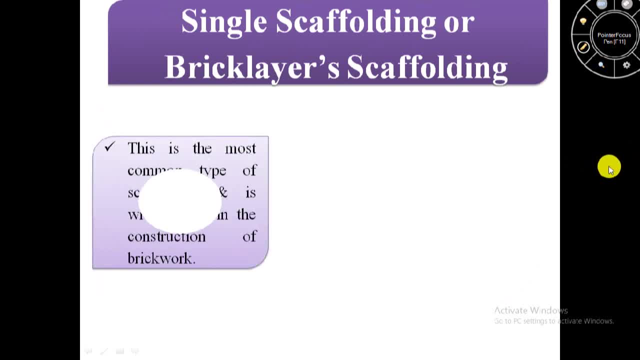 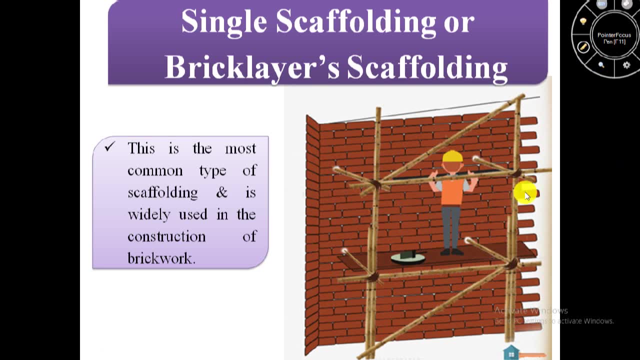 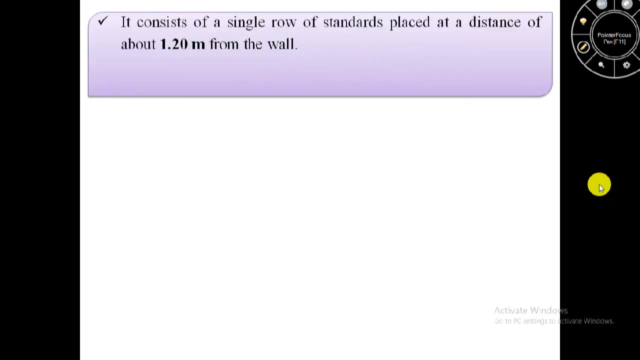 known as bricklayer scap folding. So this single scap folding is the most common type of scap folding and it is widely used in the construction of brickwork. So here this image shows single scap folding which is used in the construction of brickwork. Single scap folding consists of a. 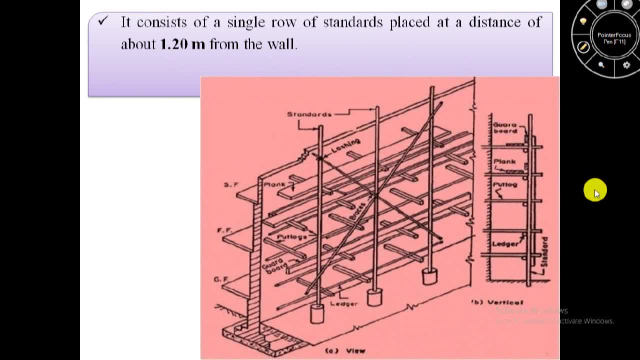 single row of standards placed at a distance of about 1.2 meters. So in this image we can see this is wall and here this single scap folding consists of single row of these standards and distance between this wall and standard is about 1.2 meters. Similarly, the 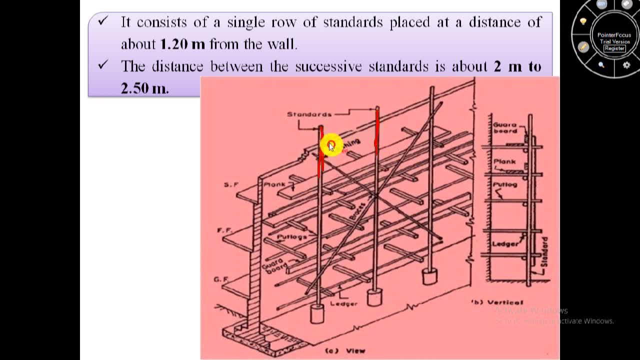 distance between these 2 successive standard is about 2 meter to 2.5 meter. In this image we can see this is wall and here this is schedule from the wall to han超2 meter. In this image we can see these are ledgers and these ledgers are fixed to these standards. 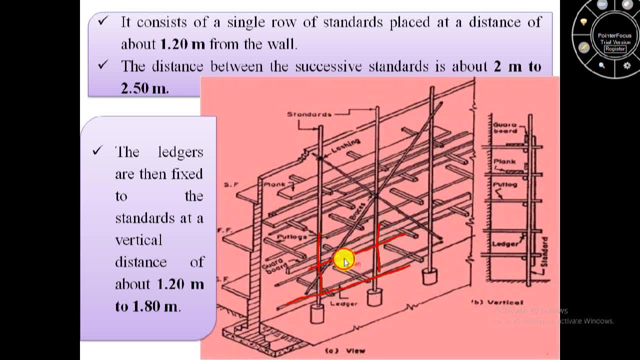 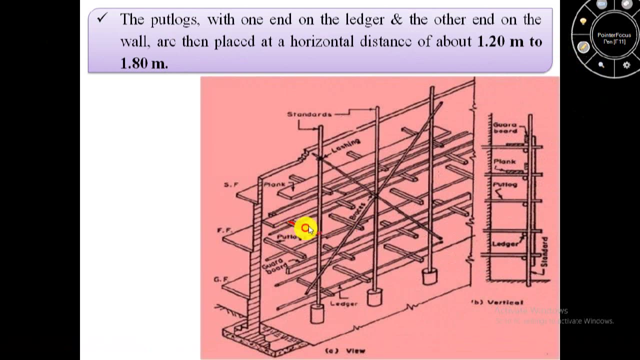 So here successive distance between vertical distance between these two ledgers is about 1.2 meter to 1.8 meter. In this image we can see here put logs are provided. These all are the put logs. So one end of this put log is on this ledger and other end on the wall. 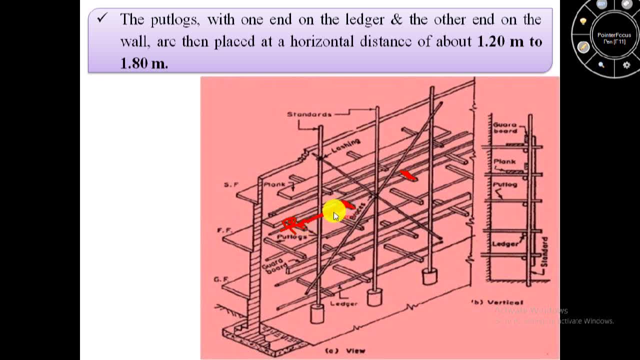 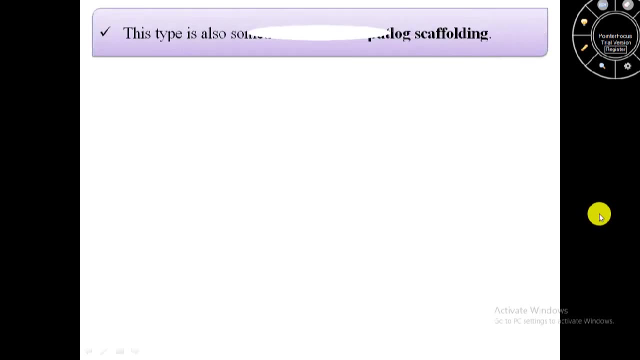 And the horizontal distance between these two put log is about 1.2 meter to 1.8 meter. Similarly, in this image we can see the braces, guard rail and toe boards are fixed. This single-scap folding is also sometimes known as put log. 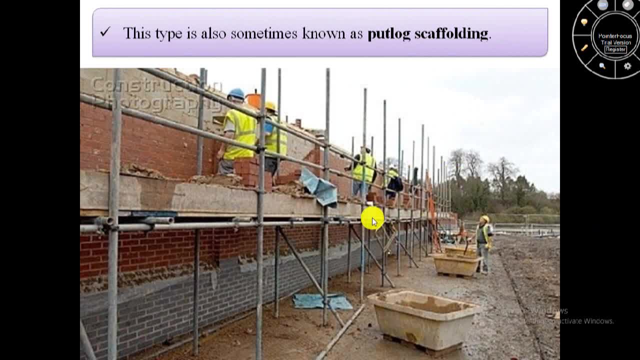 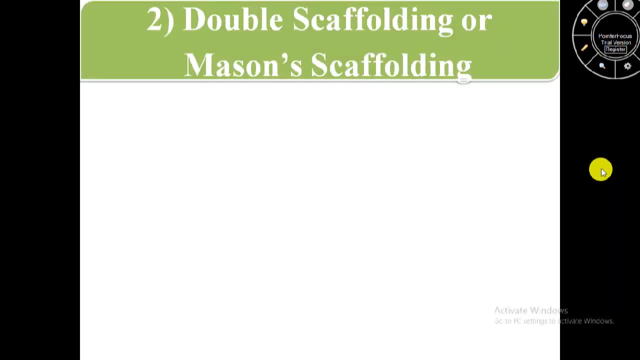 So this single-scap folding is also sometimes known as put log. This image shows actual image of single-scap folding or put log-scap folding. Now next type of scaffolding is double-scap folding, which is also known as Mason's-scap folding. 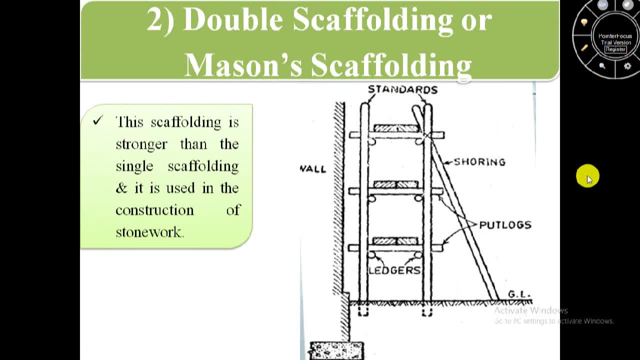 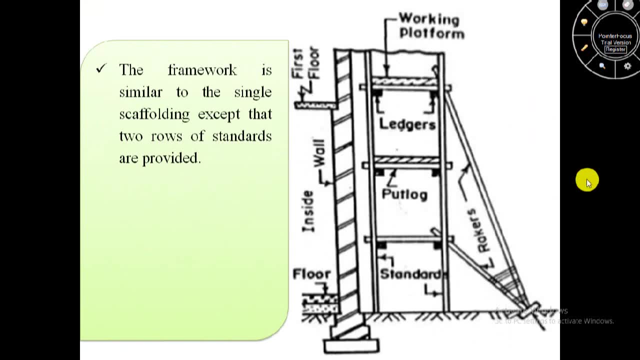 So this double-scap folding is stronger than the single-scap folding and it is widely used in the construction of stonework. The framework of this double-scap folding is similar to the single-scap folding, except that two rows of standard. 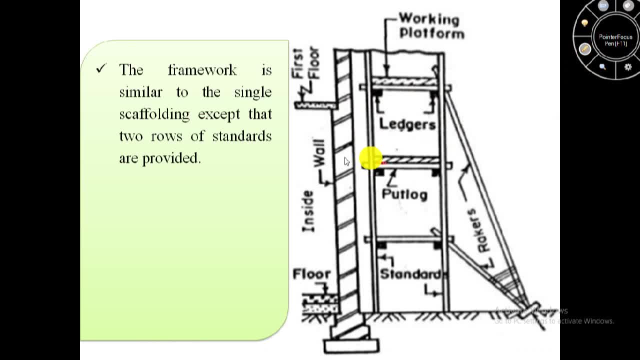 So here we can see, this is image of double-scap folding, and here this we can see: this is one, this is first standard and this is second standard. so in this double-scap folding, two rows of standards are provided. 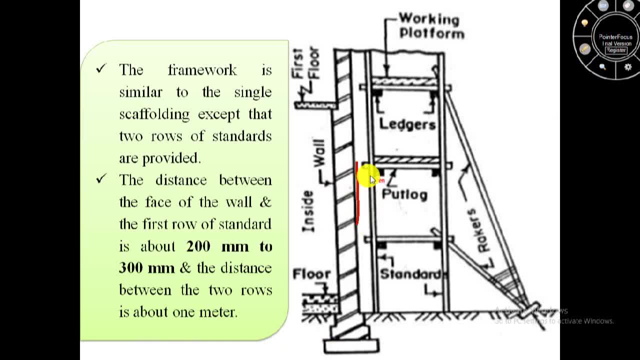 The distance between this face of wall and the first row of this standard is about 200 mm to 300 mm, And distance between this face of wall and the first row of this standard is about 200 mm to 300 mm, And distance between 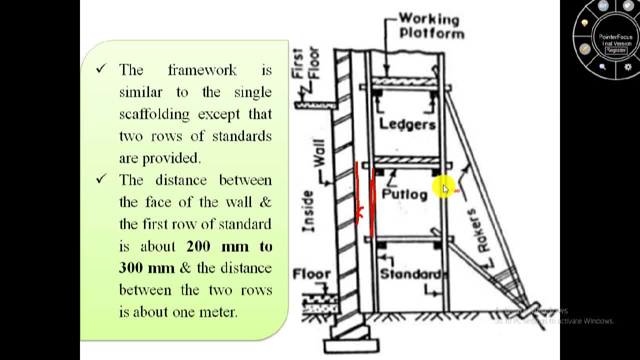 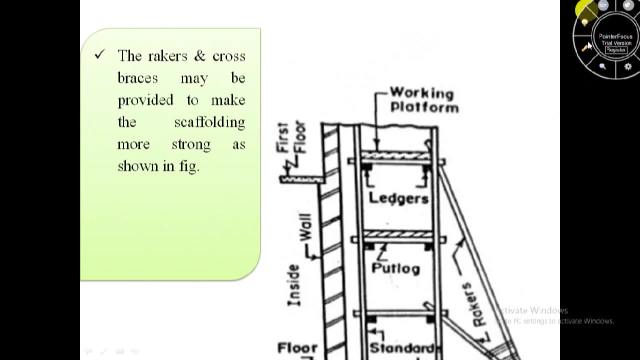 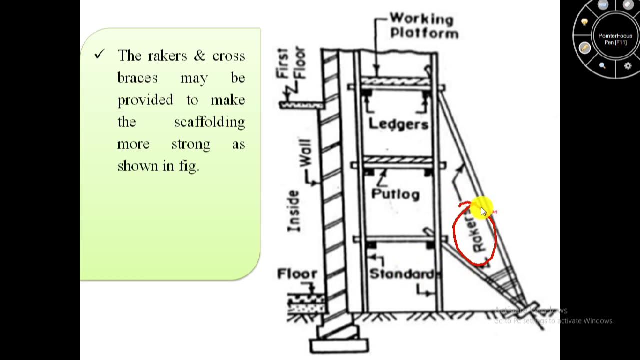 first standard and this second standard, that is, distance between these two rows of standard, is about 1 meter. In this image we can see here rackers are provided. So rackers and cross braces may be provided in this double scaffolding to make this scaffolding more strong, as shown in. 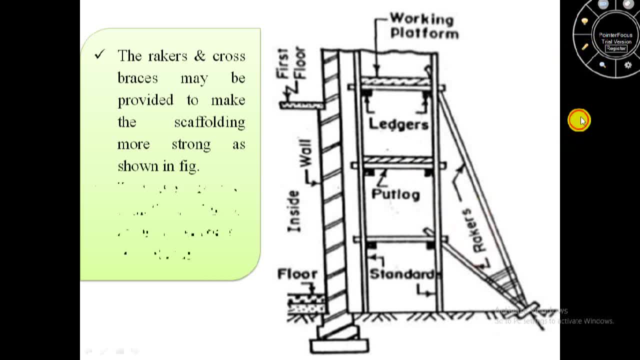 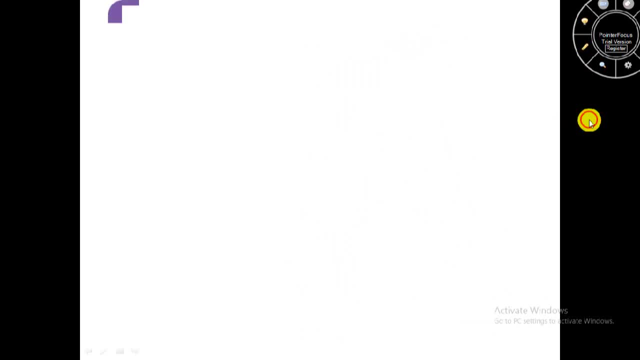 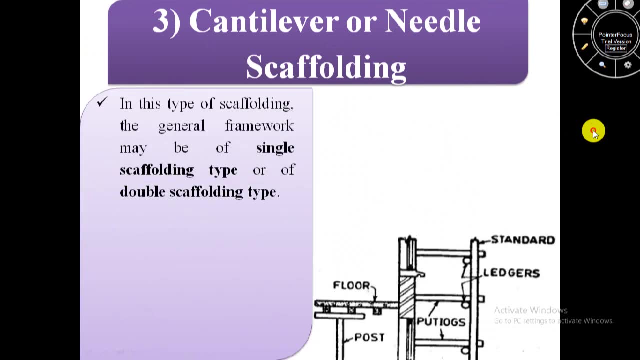 this image. This type of scaffolding is sometimes also known as an independent scaffolding. Now next type of scaffolding is cantilever or needle scaffolding. So in this cantilever type of scaffolding the general framework may be of single scaffolding type or of double scaffolding. 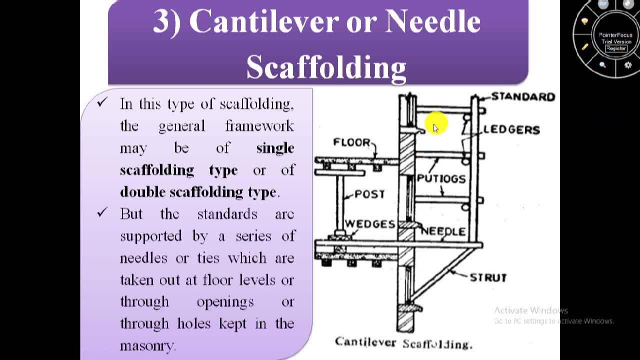 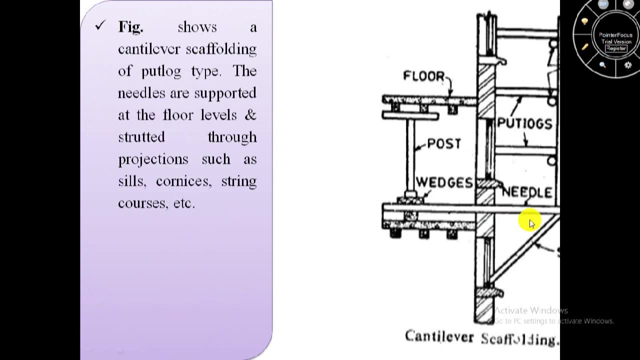 type. But here standards are supported by a series of needles- Oh Yeah, Yeah- or ties which are taken out at floor levels or through openings, or through holes kept in the masonry. Here we can see- this figure shows a cantilever scaffolding of put log type. 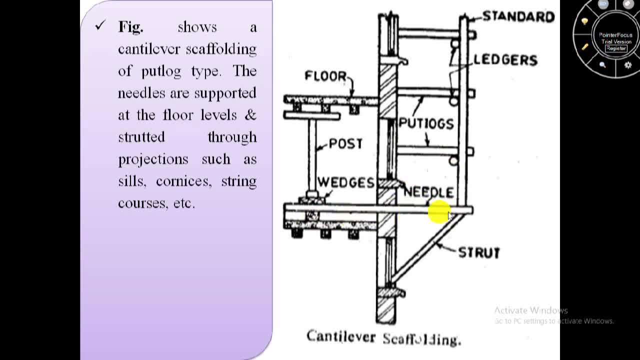 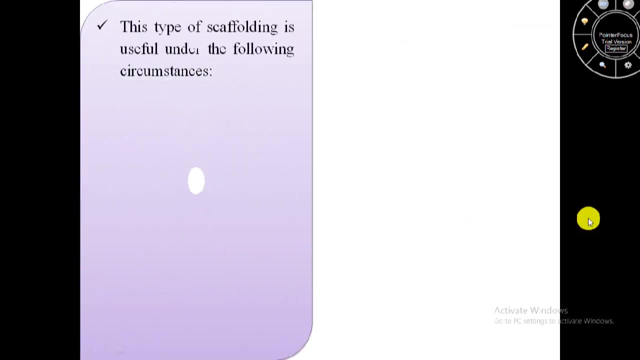 Here we can see these needles are supported at these floor levels and strutted through projections such as seals, cornices, string courses, etc. The inner end of this needle projects sufficiently inside and well strutted between the floors, as shown in this image. This cantilever type of scaffolding is useful under the following circumstances: 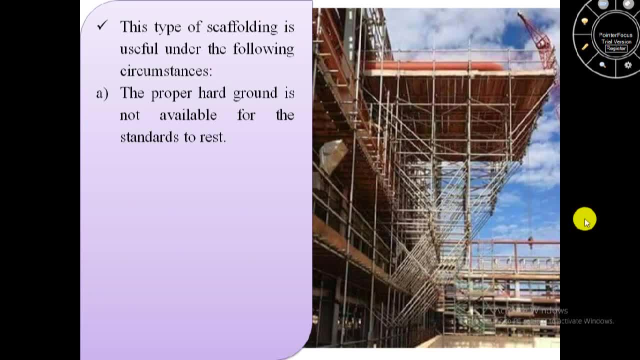 First one is the: when proper hard ground is not available for the standards to rest, at that time cantilever scaffolding is used. It is desired to keep the road or pavement straight If near the face of wall clear or obstruction caused by the scaffolding. at that time cantilever 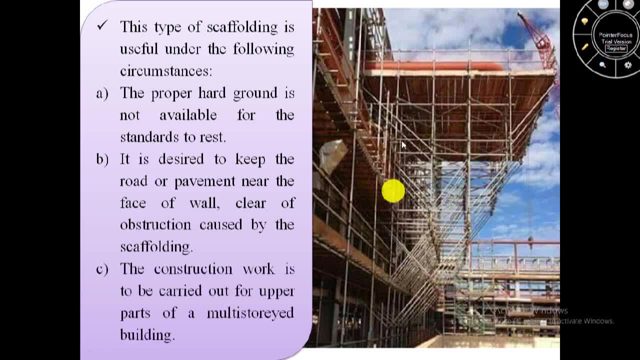 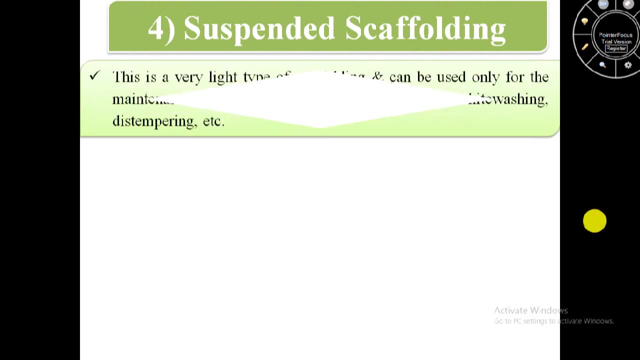 scaffolding is used. So this image shows actual cantilever scaffolding. The construction work is to be carried out for proper parts of a multi-storied building. At that time also, cantilever scaffolding is used. Now next type of scaffolding is suspended scaffolding. 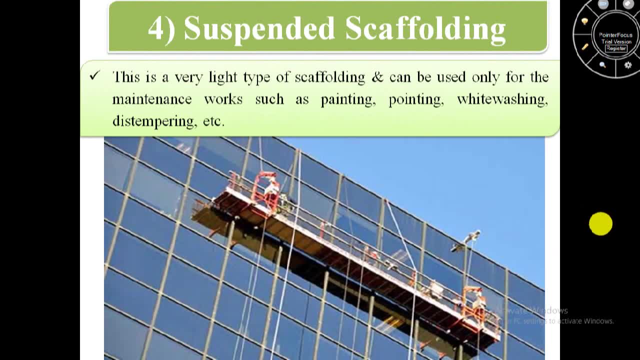 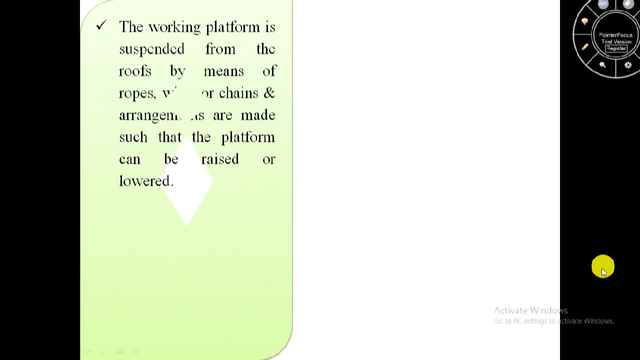 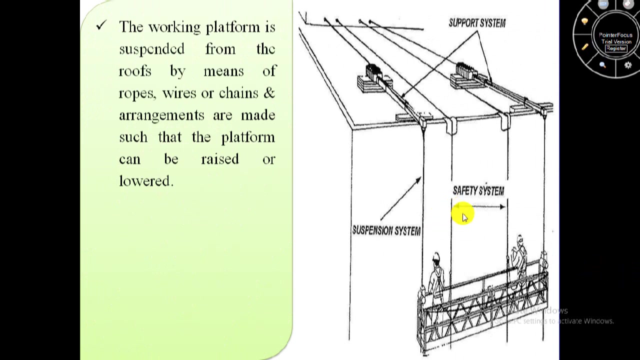 So this suspended scaffolding is very light type of scaffolding And it can be used only for the maintenance works such as painting, pointing, white washing, distempering, etc. So this image shows suspended scaffolding. The working platform is suspended from the roofs by means of ropes, wires, chains and 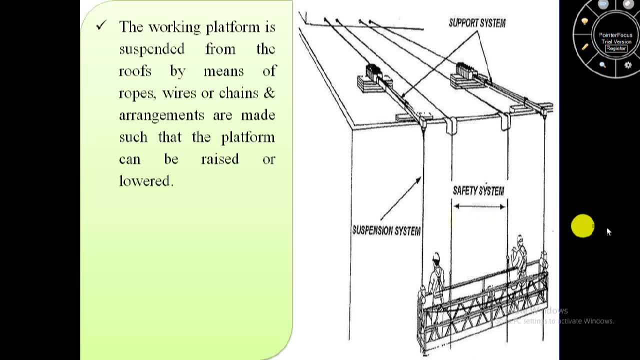 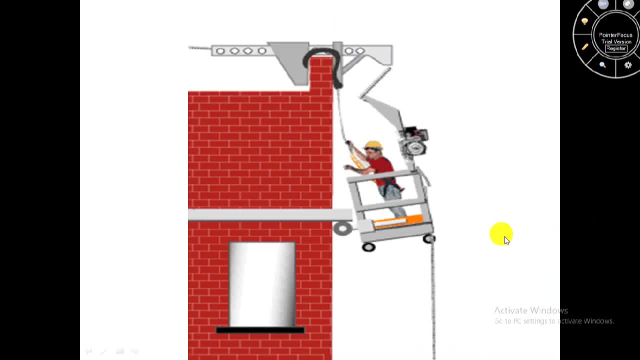 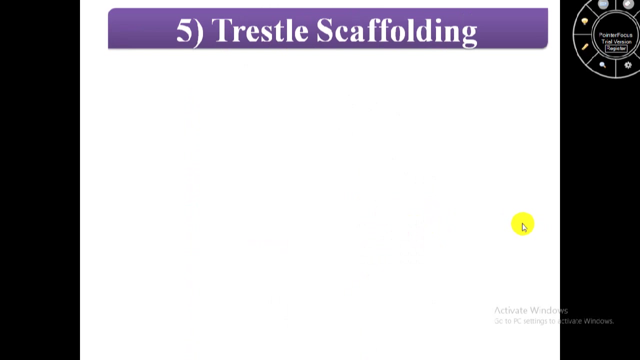 arrangements are made such that the platform can be raised or lowered. This suspended type of scaffolding does not create any problems And it is most effective, as it always provides the optimum level of working. Here we can see actual working of suspended scaffolding. 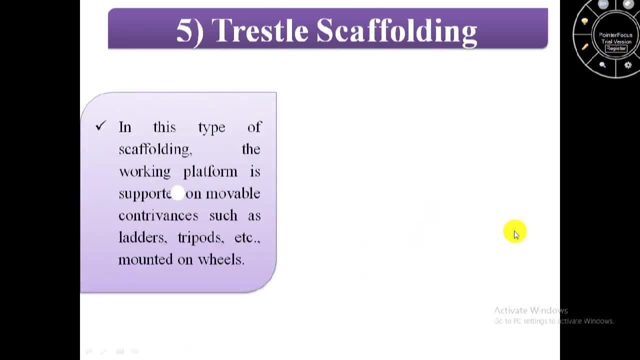 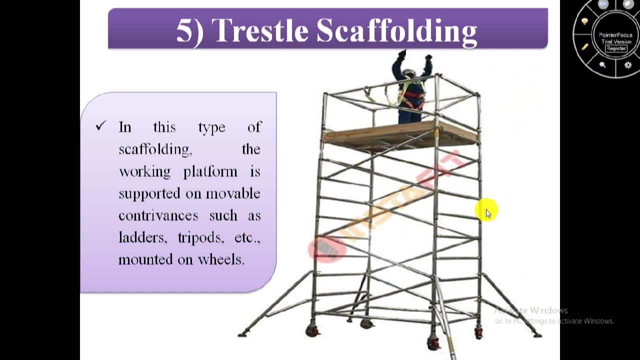 Next type of scaffolding is trestle scaffolding. So in this type of scaffolding the working platform is supported on movable contrivances such as ladders, trippers etc. mounted on wheels. So in this image we can see this is a working platform. 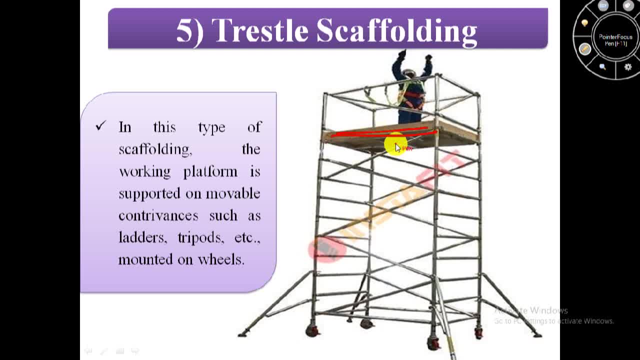 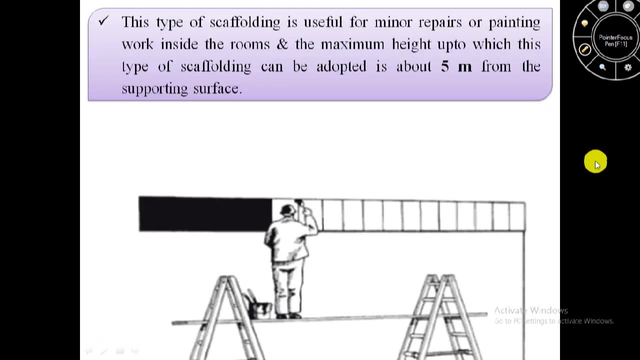 And this working platform is supported on the movable contrivances such as ladders, trippers etc. mounted on these wheels. So this one is trestle scaffolding. This trestle type of scaffolding is useful for minor repairs or painting work inside. 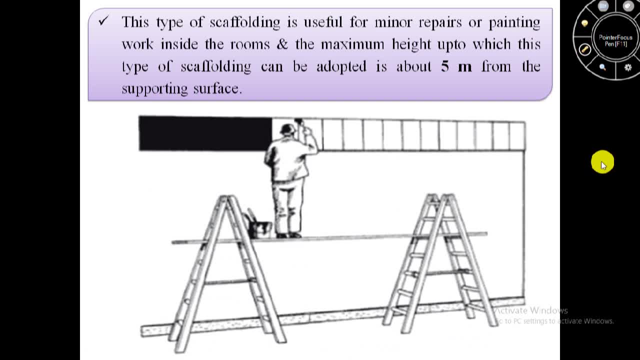 the room and the maximum height up to which this type of scaffolding can be used. So in this image we can see this is a working platform And this working platform is supported on the movable contrivances such as ladders, trippers, etc. 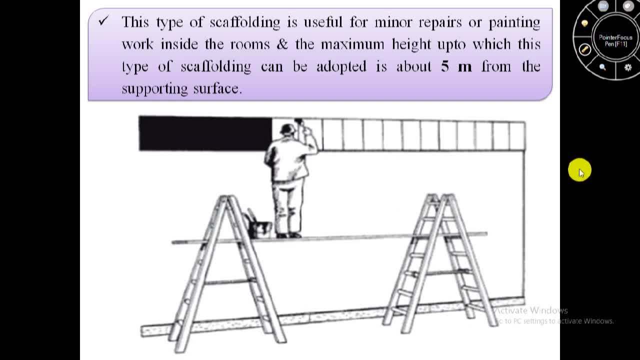 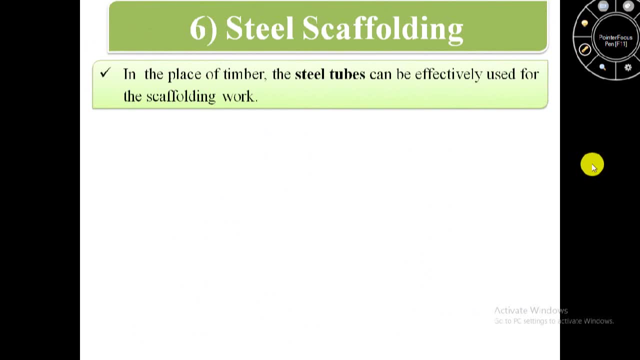 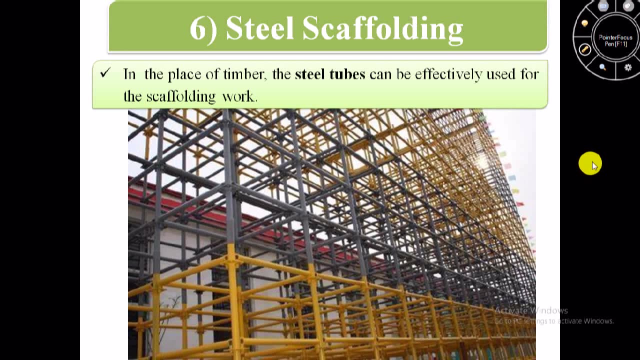 can be adopted is about 5 meter from the supporting surface. Now next type of scaffolding is steel scaffolding In the place of timber. the steel tubes can be effectively used for the scaffolding work. and these are the steel scaffolding The diameter: 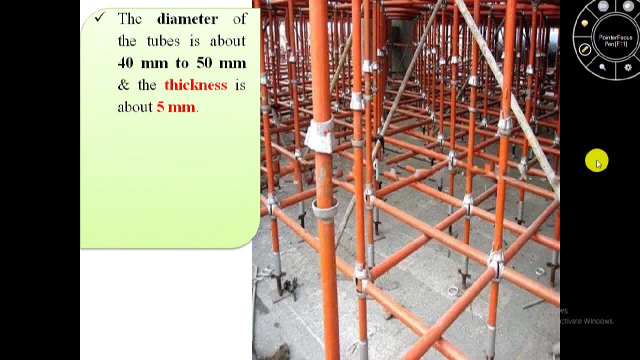 of the tubes used in the steel scaffolding is about 40 mm to 50 mm, and the thickness of these tubes is about 5 mm. These tubes are available in standard lengths with special couplings and set screws. This image shows steel scaffolding. The advantages of steel. 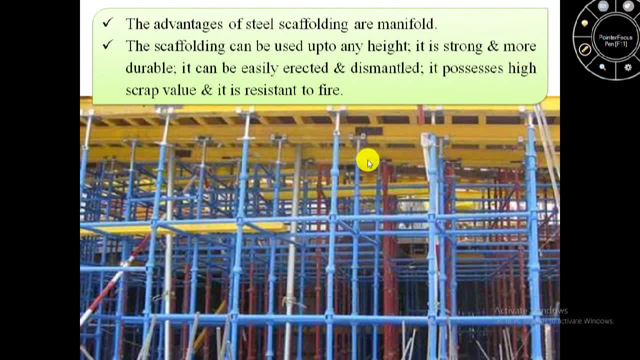 scaffolding are manifold. The scaffolding can be used up to any height. This steel scaffolding is strong and more durable and it can be easily erected and dismantled. It possesses high scrap value and is very durable. It is resistant to fire. However, the disadvantages are that the initial cost is high. It requires 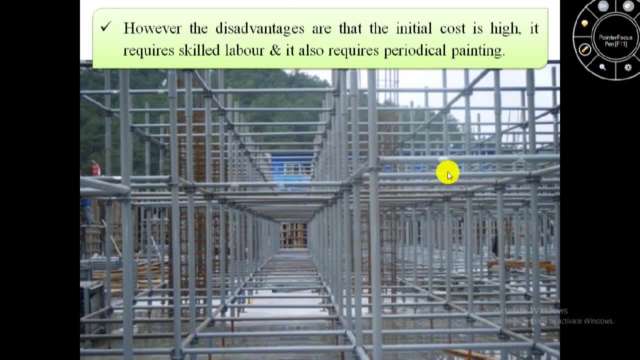 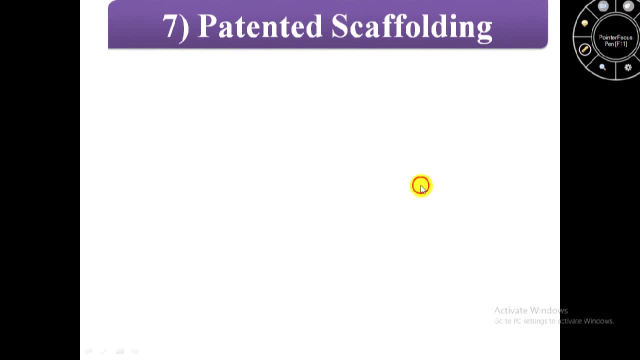 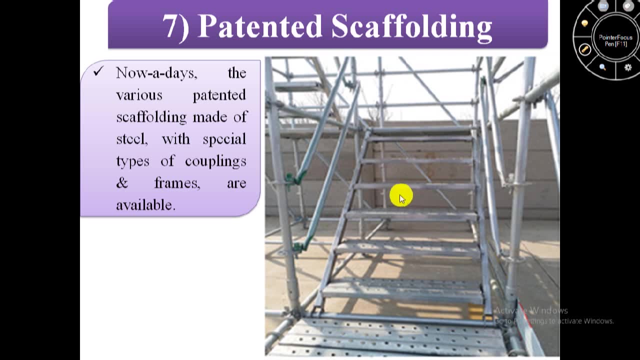 skilled labor and it also requires periodical painting. Now next type of scaffolding is patented scaffolding. This is the last type of scaffolding. So nowadays, the various patented scaffolding made of steel with special types of couplings and frames are available. 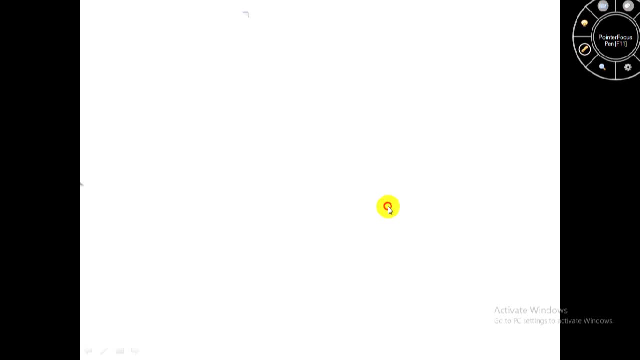 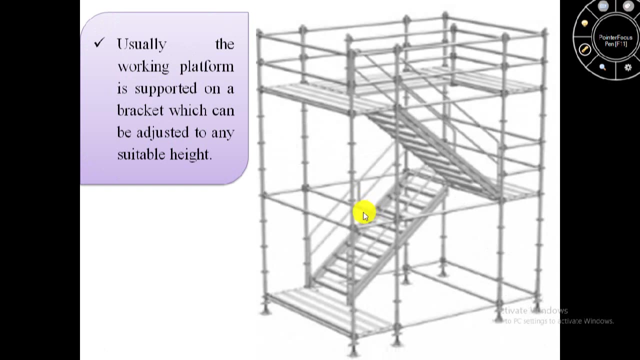 So this image shows patented scaffolding. Usually, the working platform is supported on a bracket which can be adjusted to any suitable height. So we can see this is the patented scaffolding and in this patented scaffolding, this working platform is supported on a bracket which can be adjusted to any. 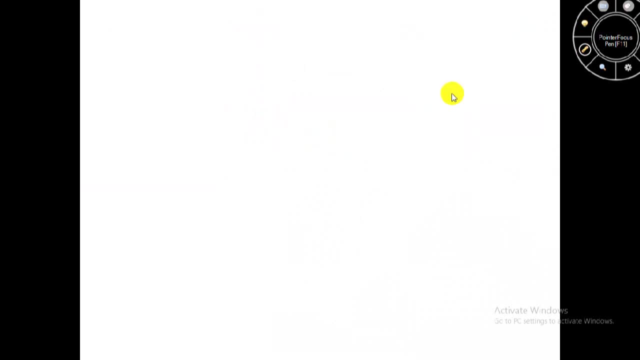 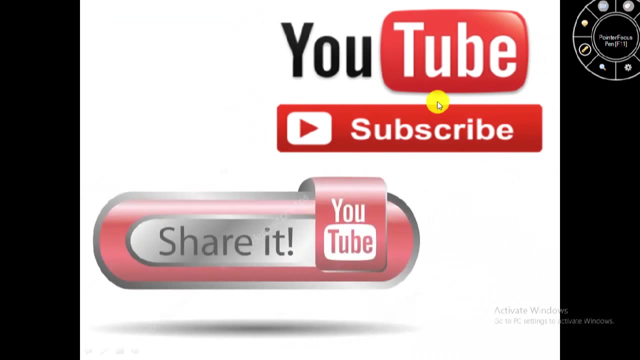 suitable height. So here this video is finished. I hope this video will be helpful for you. For more updates, subscribe my channel and don't forget to share this video with your friends and family. Thanks for watching. Please share this video with your friends and family.